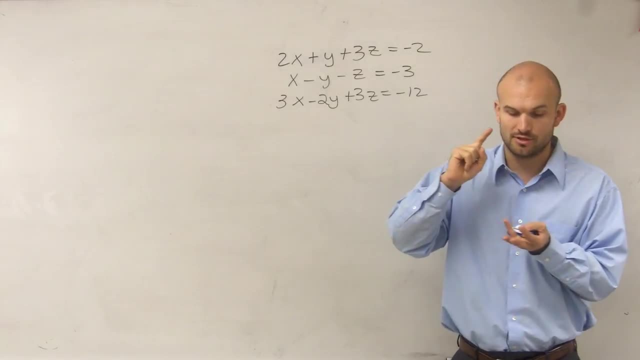 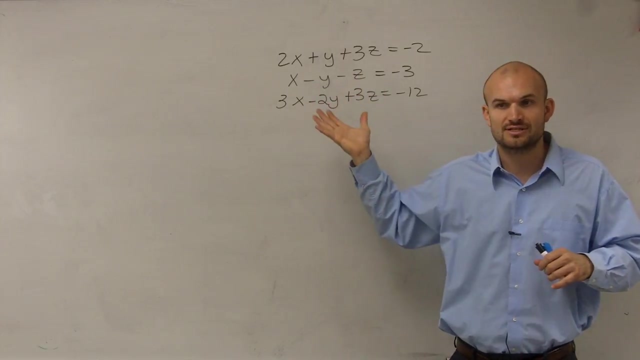 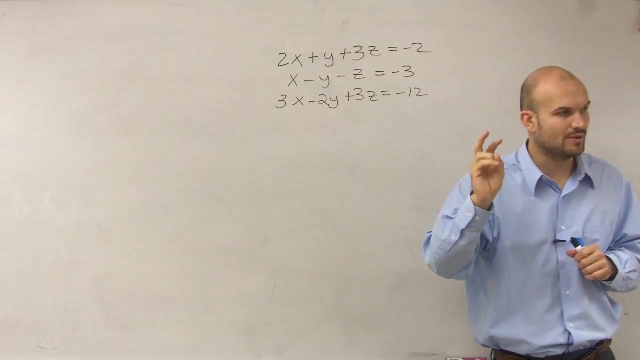 We learned elimination, substitution, and we also learned graphing right. So our main goal is, if we can take this system of three equations and break it down to a system of two equations with two variables, all right. So to get it down to two equations and two variables, what we first need to do is get rid of a variable. 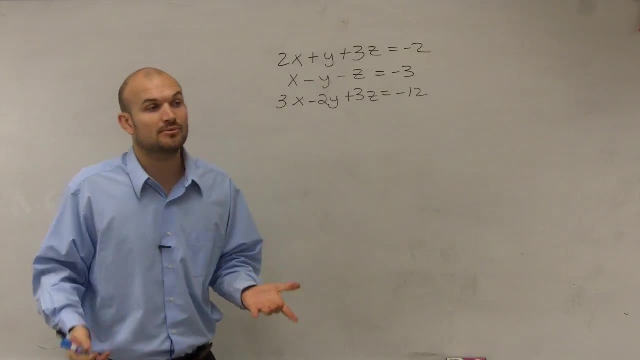 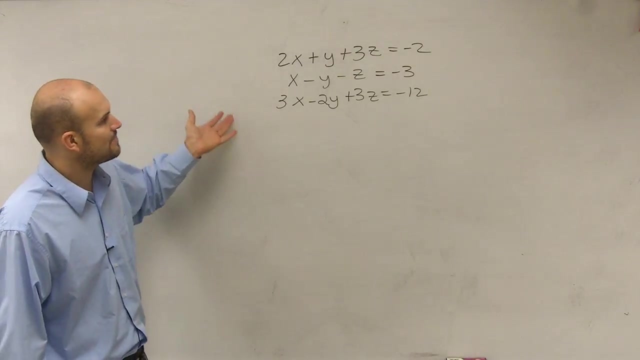 And remember just when we learn the elimination technique, the best variable to get rid of is one that has a coefficient of one or negative one. And so we look at here and we look at where is there a variable that we have a coefficient of one or negative one? 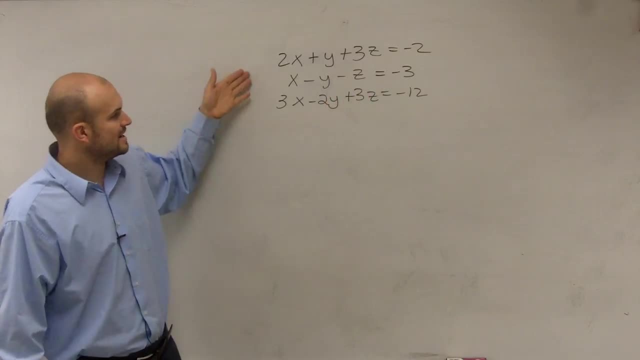 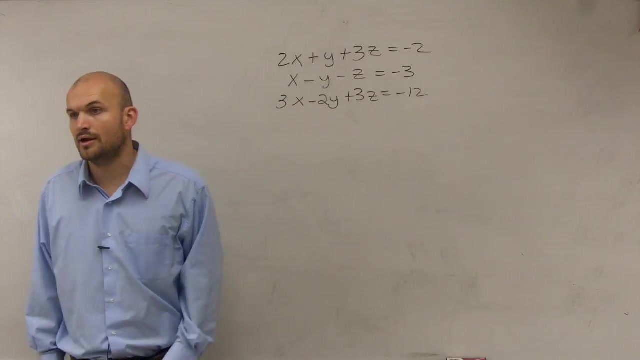 X, Y and also Z. right Now, I would probably say that the variable with a one compared to a negative one would probably be the easiest to get rid of. all right, And actually did I already go over this problem with you guys? 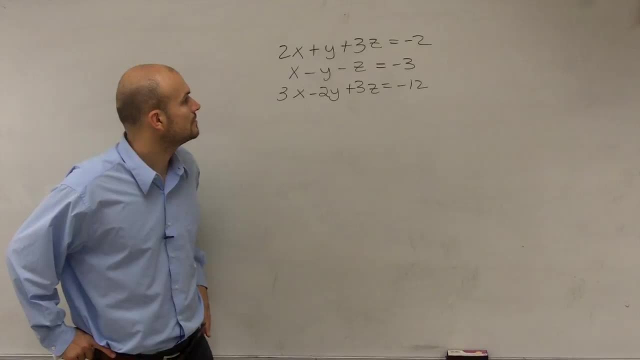 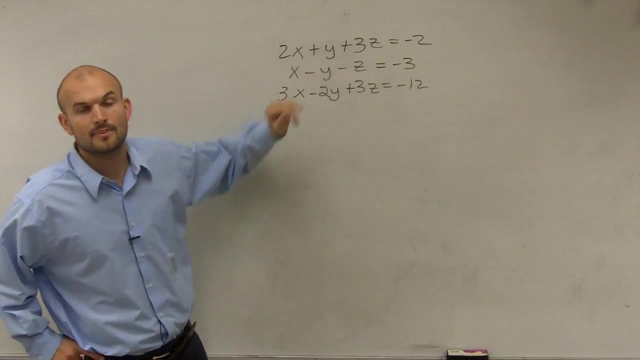 Maybe it was the alone, I'm sorry. Right, okay, You're right, So you could get. so, to get rid, so I could get rid of a Y very quickly with this one, right, Right, But maybe someone wants to get rid of X. 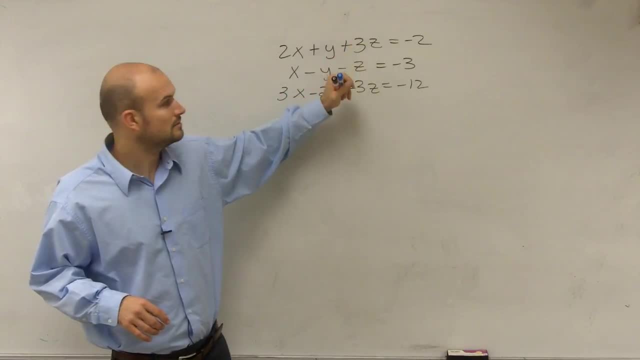 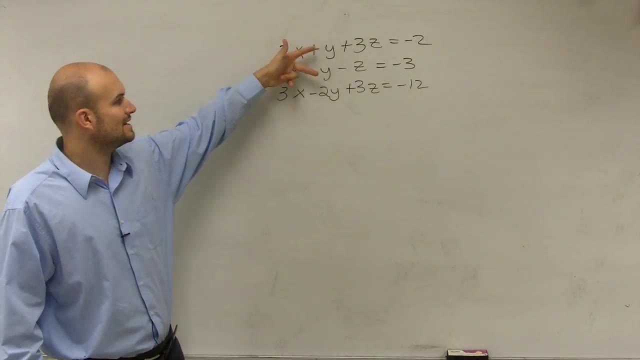 Did anybody do Z? Nobody. Oh, I did Z with the three and the other three. Okay, Yeah, you could do Z with the threes, I would probably say, even though, yes, you could probably get rid of the two Ys. 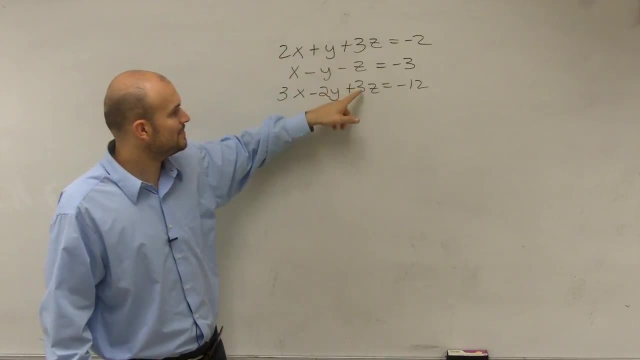 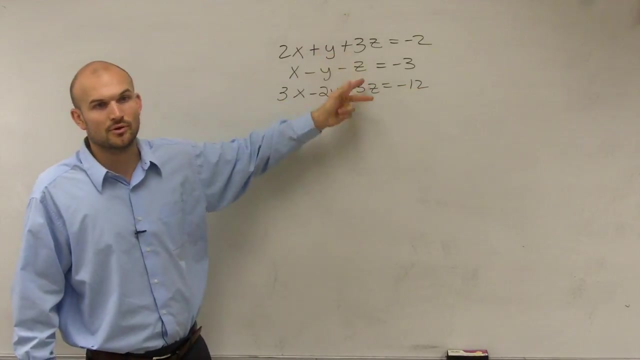 by adding them, these two equations, up. this one might be the easiest to get rid of the Zs, because all I have to do is multiply this second equation by three and add it to both of those equations. Does everybody see that? 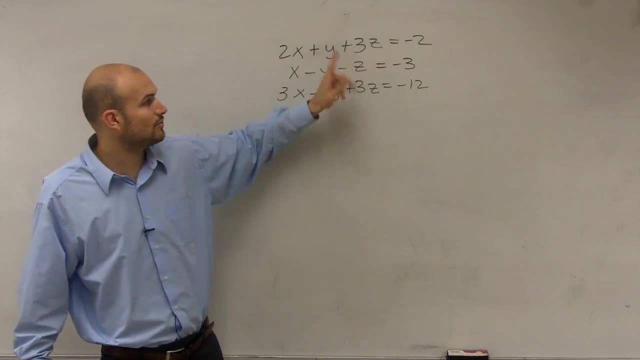 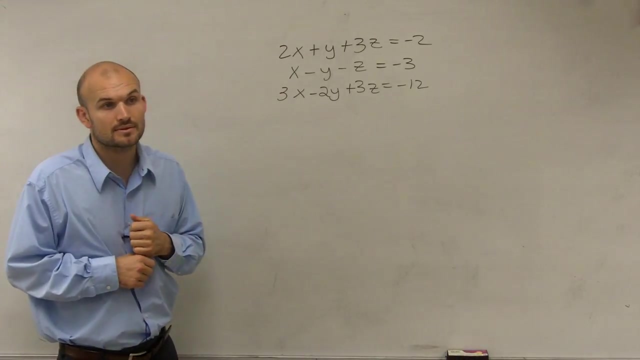 It doesn't really matter which way you guys go, though. You can eliminate the X, the Y or the Z, It does not matter. Let's actually go through this one. I'm sorry, You want me to eliminate the X. 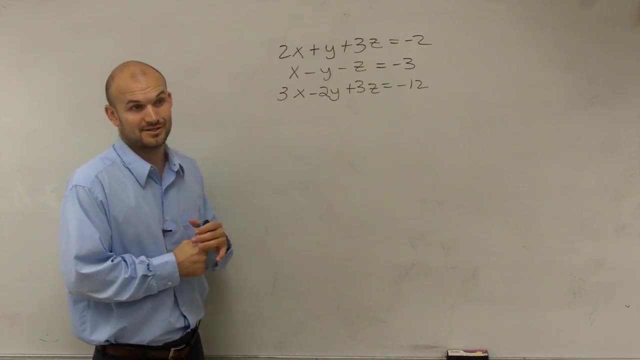 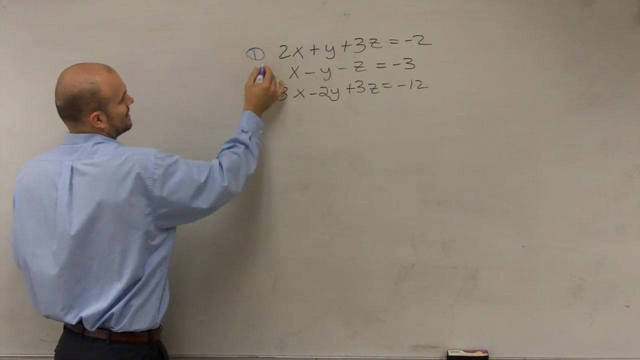 I actually already recorded one for solving for the X, so I'm not going to solve for the X, Let's do the Z. That actually sounds like a good one. So the first thing I like to do is label them: one, two and three. 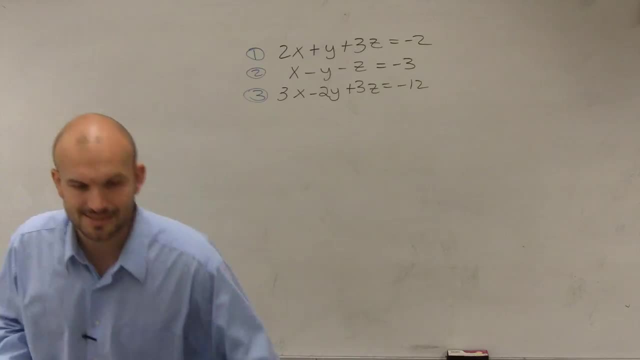 All right. So what I'm going to do is I need to pick two equations to eliminate the Z, So I'm going to eliminate this. I want to eliminate my Z variables, So what I'm going to do is I'm going to take equation. 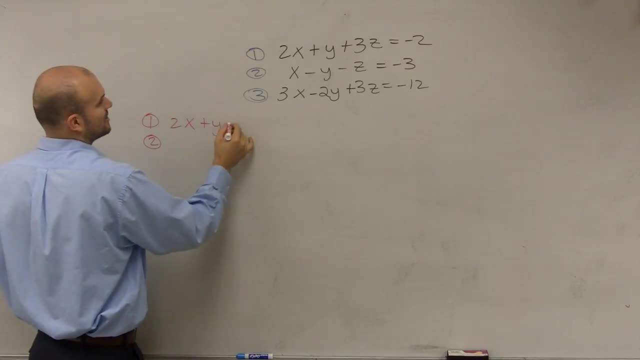 equation number one and equation number two. So I have 2X plus Y plus 3Z equals negative two. and then I have X minus Y minus Z equals negative three. Then I'm going to take equations, I'm going to take equation number one, two and three. 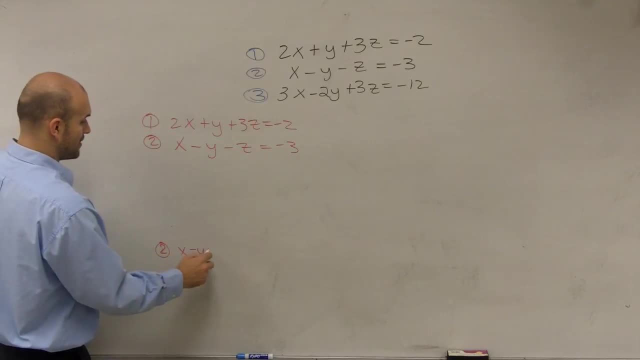 So two would be X minus Y minus Z equals negative three, And equation three would be 3X minus 2Y plus 3Z equals negative 12.. Now does anybody know why I chose equation number one and two and two and three? 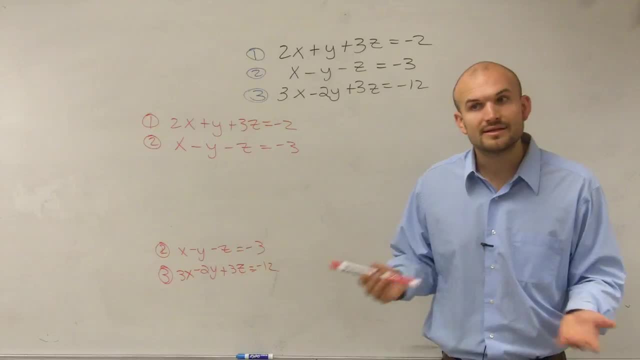 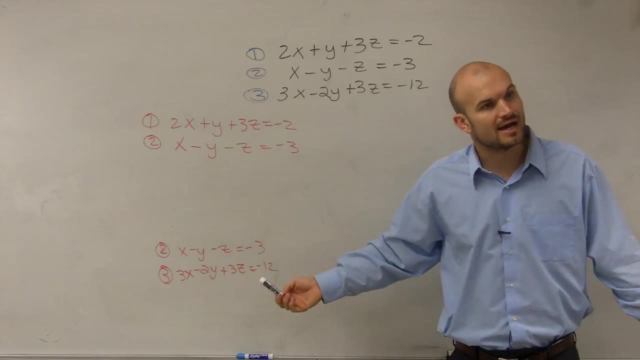 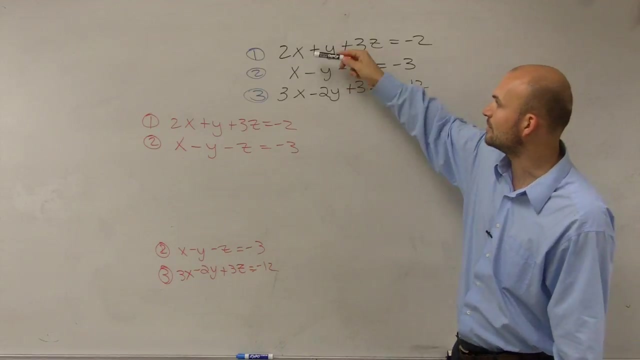 Could I pick different equations? Yeah, It doesn't. it's okay which ones you want to pick. If you guys wanted to do equation one and two and then do equation one and three, that's fine. If you guys wanted to do one and two and then two, or well. you can't do two back one. 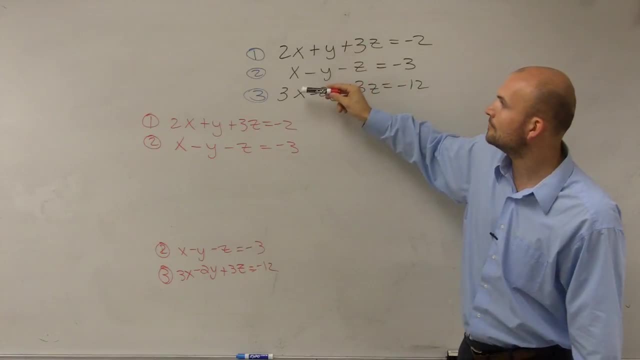 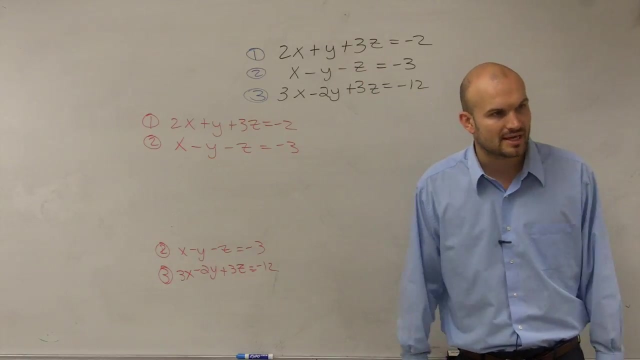 but if you could do one and two and then one and three, Or you could do two and three and then two and one, which we did up there. So it's okay which way you pick it, But the main important thing is we need to eliminate our variable. 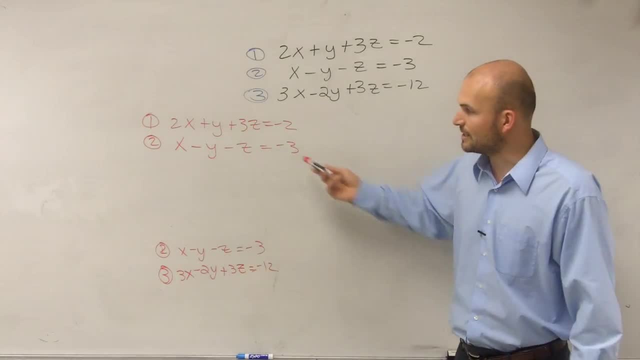 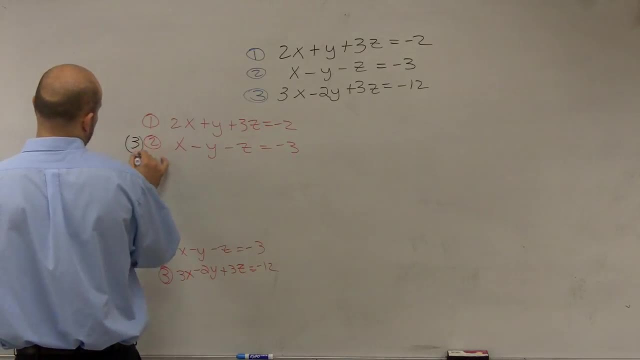 Now, we've talked about this. We've talked about this. We've talked about this. So the easiest way to eliminate variable Z is to multiply equation two by our multiplier three. So that's exactly what I'm going to do: I'm going to multiply equation two. I'll multiply it, like this, times three. 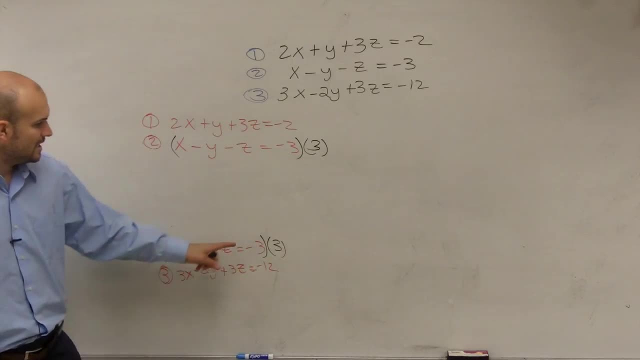 And the reason why I'm going to multiply the equation by three is because when I multiply three times negative Z, I now have a negative 3Z. All right, So let's actually just write it out what it's going to look like. 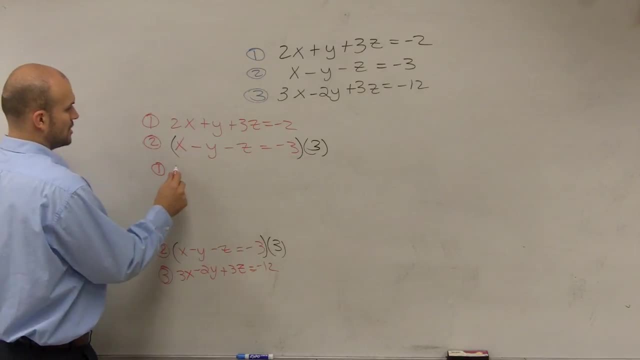 So I'm going to rewrite equation one again. So equation one is 2X plus Y plus 3Z, equals negative two. And then now my new equation two, which is now going to be 3X minus 3Y minus 3Z, equals- let's see, negative nine. 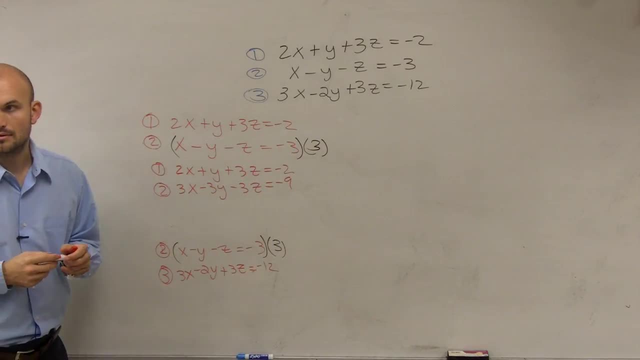 All right, Did everybody say that? So then, what we do is we add them by elimination. Since I have a positive and a negative of the same coefficient, I'm going to add them Here. I get 5X minus 2Y. 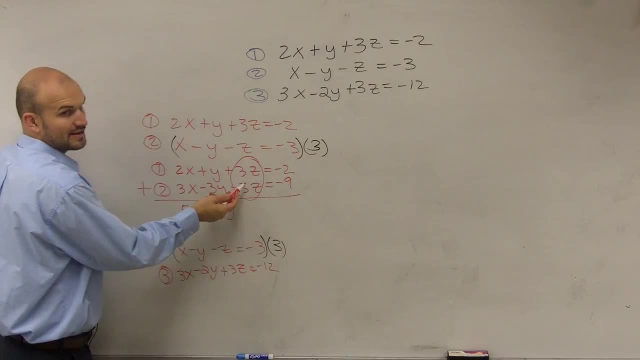 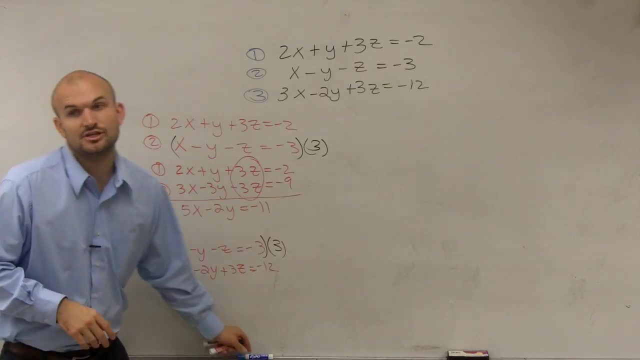 This goes to zero or adds to a zero as a coefficient. Zero times Z is zero, And then this gives me negative 11. So that new equation only has how many variables? Two, Two. So I'm going to label that as A. 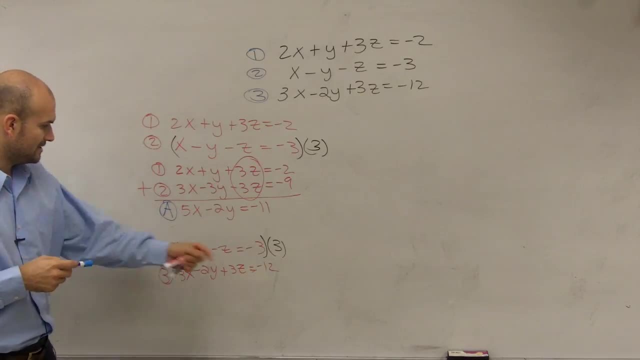 All right, Then we do the same thing. I use my multiplier, which, again, I already know. it's equation, this number 3X, So I only have to do my math once. So I rewrite equation two, which is 3X minus 3Y minus 3Z equals negative nine. 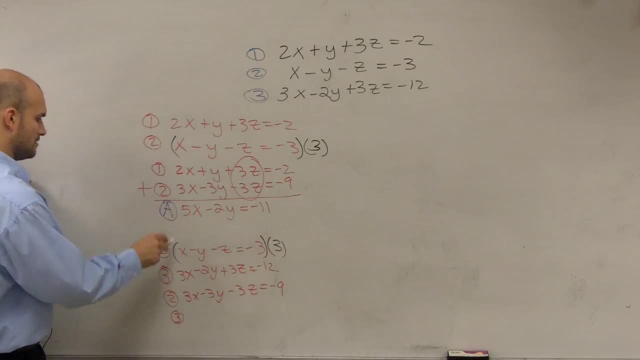 And then I rewrite equation three, which is 3X minus 3Y minus 3Z, equals negative nine. 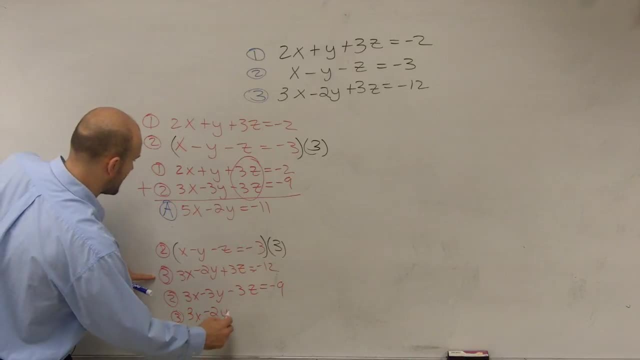 And then equation three, which is 3X minus 2Y plus 3Z, equals negative 12. And now, when I add up those two equations, I get 3X plus 3X is- let me put it in red again- 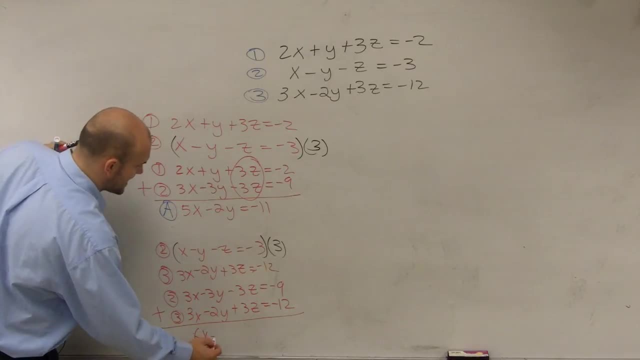 6X, This becomes negative, 5Y, This becomes zero, And that becomes negative 21.. And since now again I created another equation with two variables, I'm going to call that equation B. Does everybody follow me? Can everybody see that kind of down there? 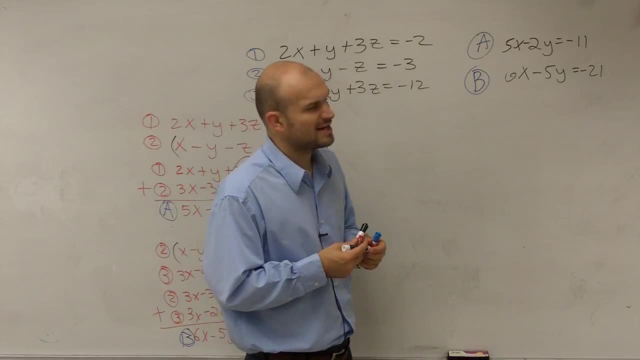 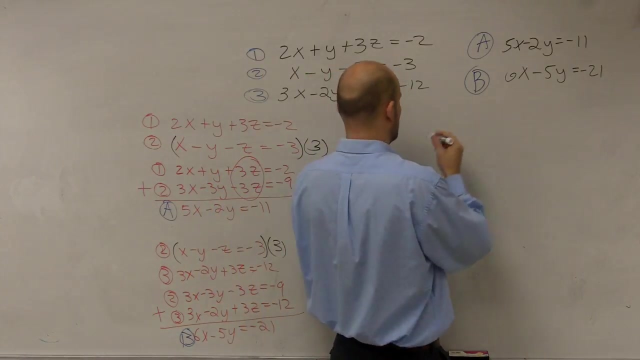 Yeah, y is probably what I'd like to do as well. So let's eliminate the y's. So to do that, I'm going to multiply my a times. let's do it by negative 5.. 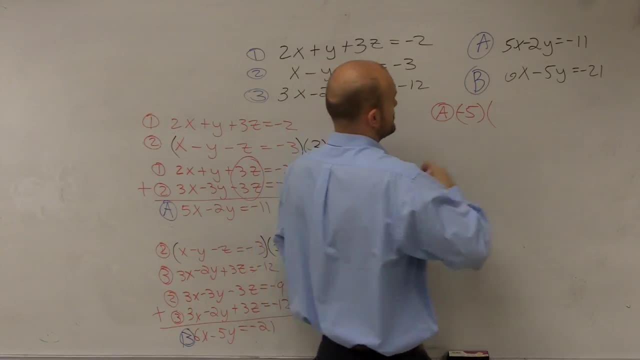 So I multiply a times a negative 5.. So that would give me a 5x minus 2y equals a negative 11.. I haven't multiplied it through yet. And then b will multiply by a positive 2.. So b will multiply by a positive 2, so that will be 6x minus 5y equals negative 21.. 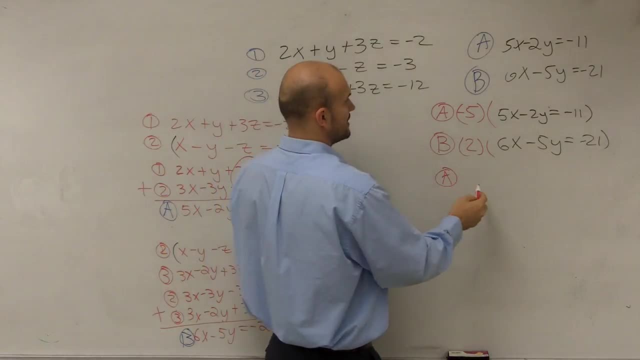 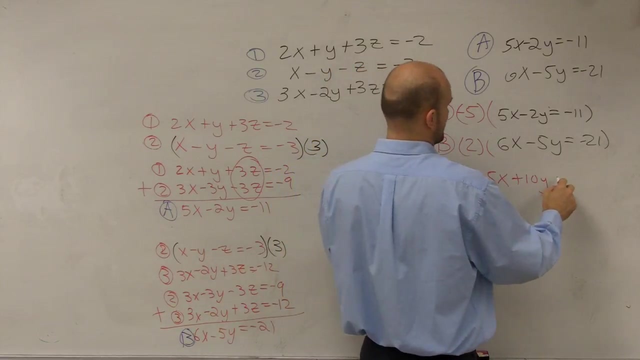 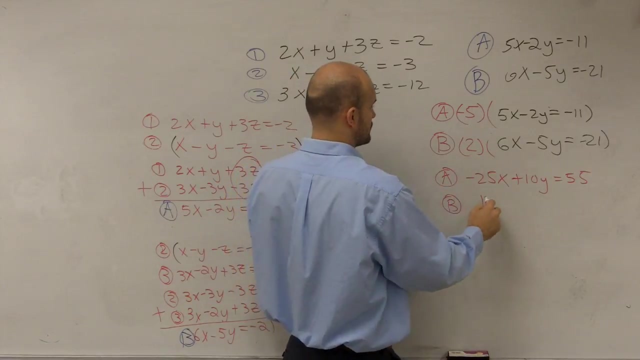 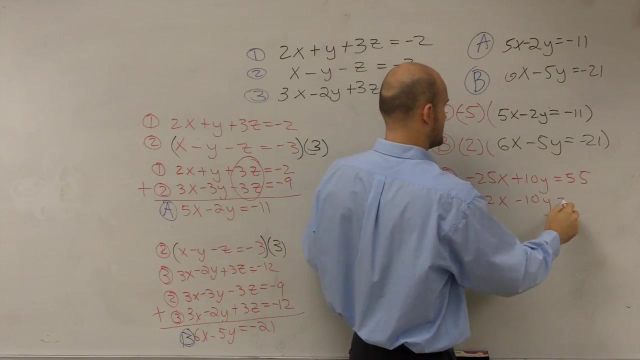 Okay. so when I multiply those through, my new a is now going to be negative 25x plus 10y, equals positive 51.. And my new b is now going to be 12x minus 10y minus, or equals negative 42.. 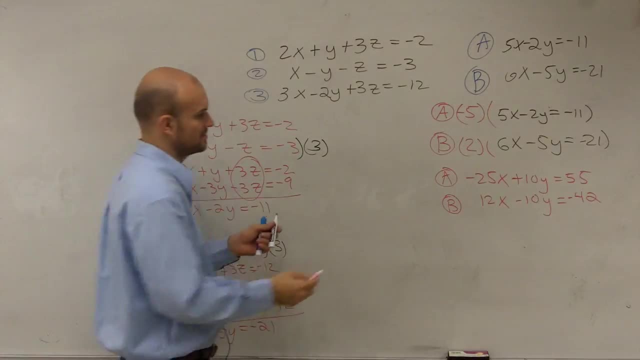 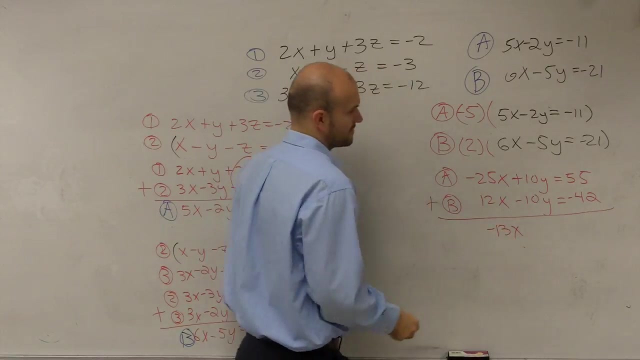 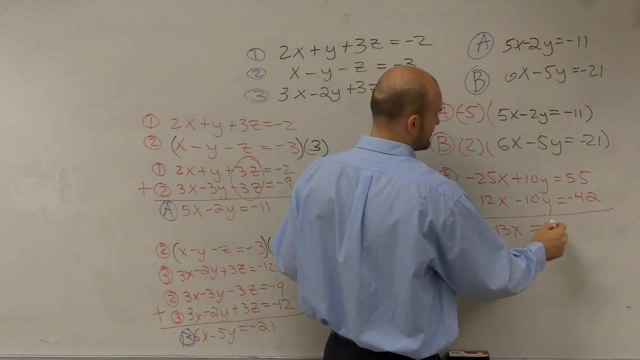 Right, We're using elimination for two variables. Add them up. This gives me negative 13x. That goes to 0. And then I'm going to multiply by a positive 12x, And then this becomes a negative positive 13.. 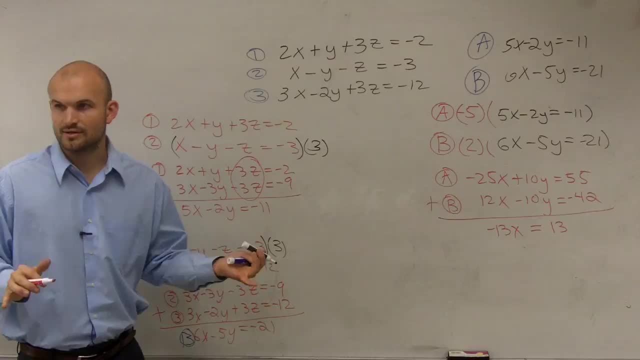 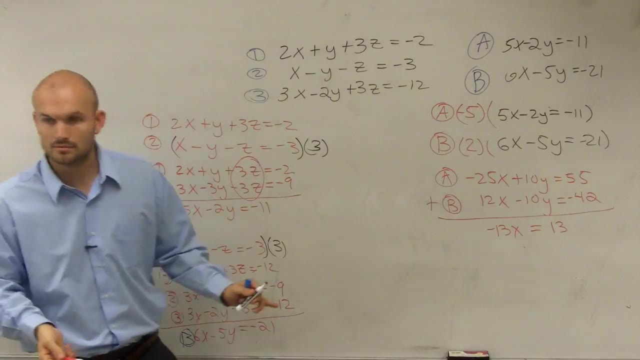 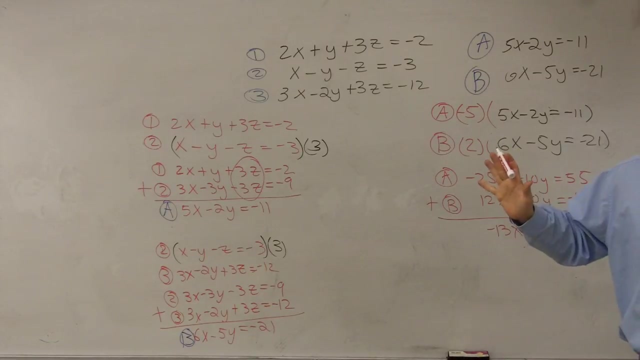 Question: No, You good. Does everybody kind of see what I'm doing? Yes question. All I'm doing is I'm doing elimination. Okay, There's multiple different ways to do it, So your work could be totally different, but you still get the right answer. 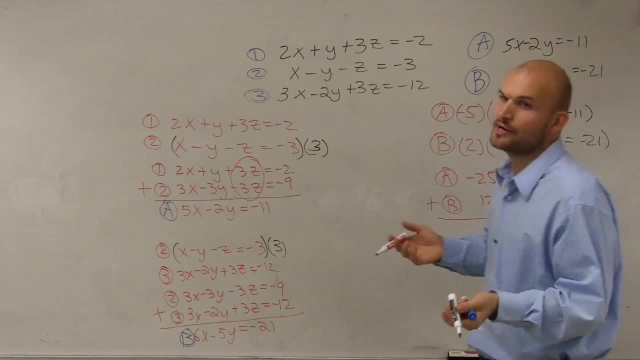 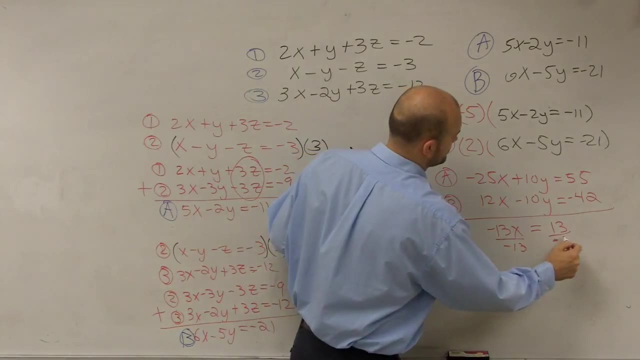 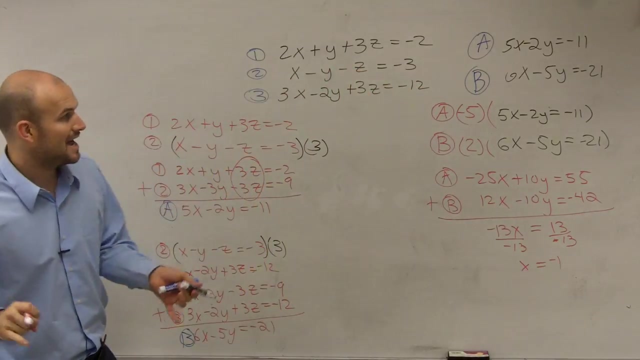 Okay, it's very possible. with a problem like this, It's very easy to mess up. So now I just divide by negative 13. X equals negative 1.. So now I know what one answer is right. So now I plug negative 1 back into one of my equations. 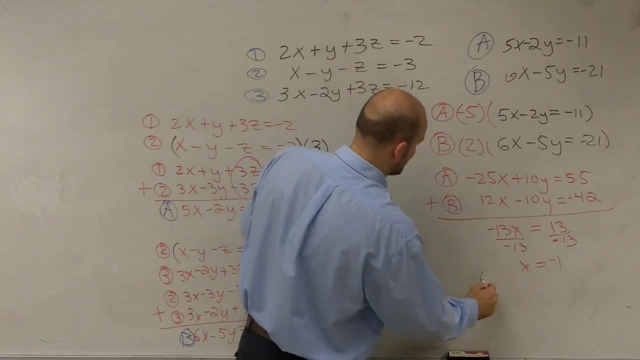 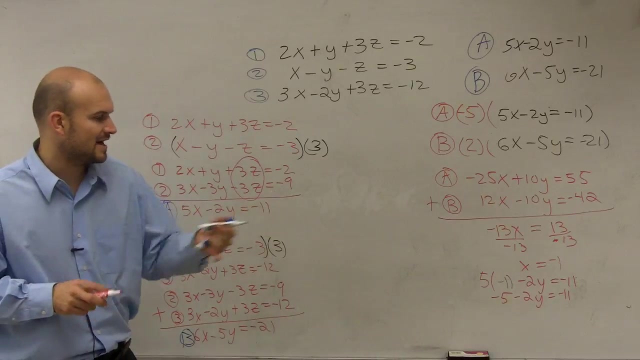 All right, So I do 5 times negative 1.. Minus 2y equals negative 11, and this gives me negative 5 equals negative. 5 minus 2y equals negative 11.. To kind of ease my work here, I'll add the 5 to the other side to get me negative 6.. 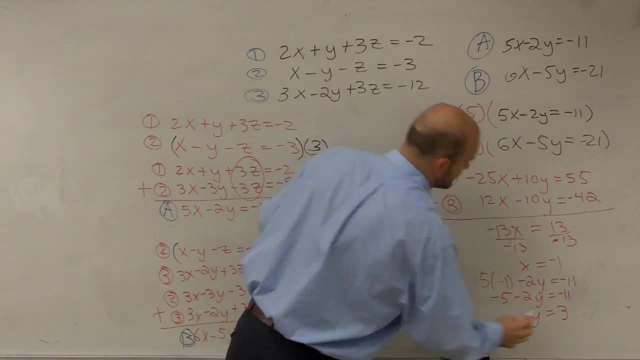 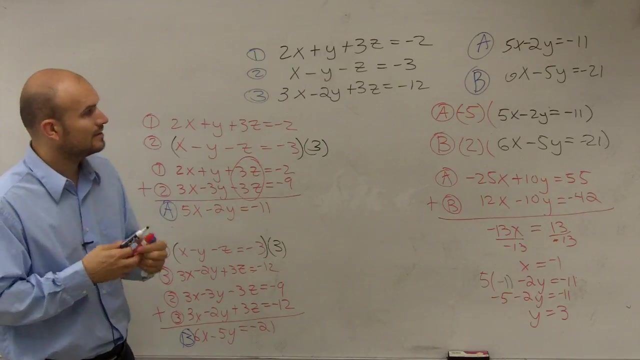 Divide by negative 2, and I get y equals positive 3.. Okay, You guys can do your work on your own. I'm just going to have to kind of move this along. So now I know y equals 3 and x equals negative 1.. 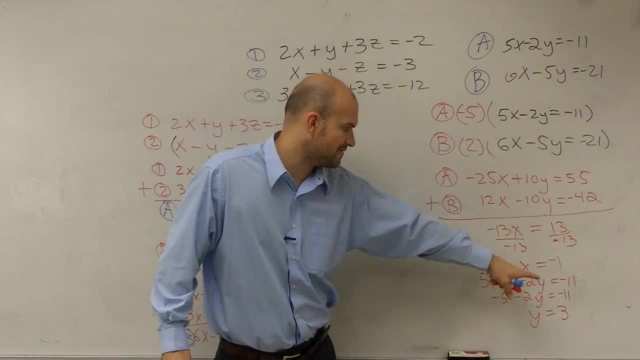 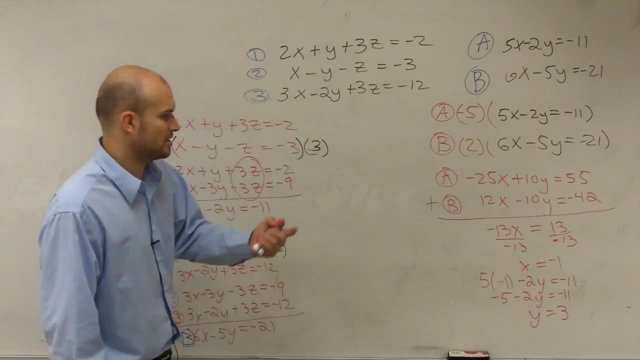 Well, if I add the 5 over there, I'm going to have negative 2y equals negative 6.. So then I divide by that, Yeah, I'll get a positive 3.. And then so the last one we just need to solve for z. 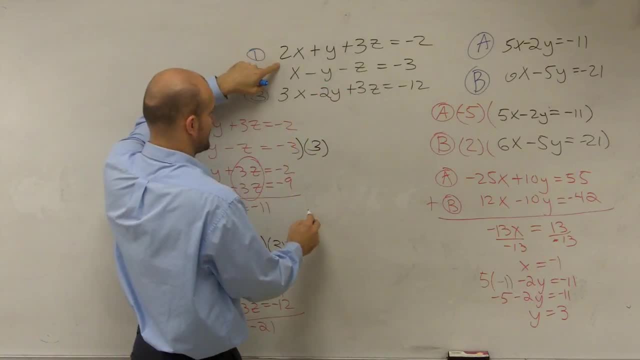 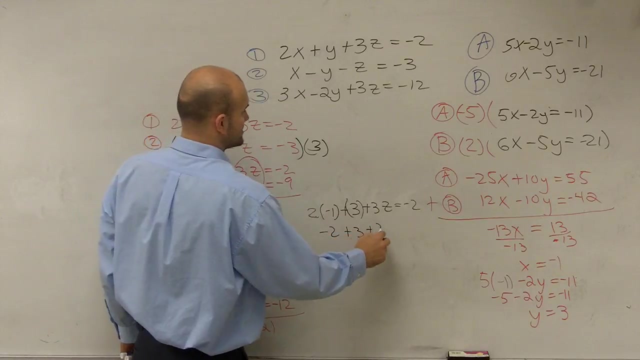 So what I'll do is: it doesn't matter again which equation you guys pick, but I know what x is, which is negative 1, plus y, which is 3, plus 3z, equals negative 3.. So you get negative 2 plus 3 plus 3z equals negative 2.. 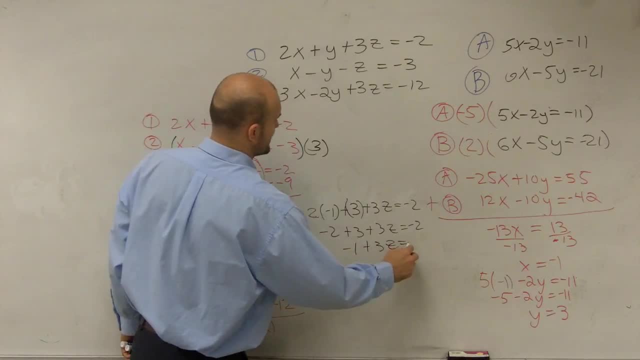 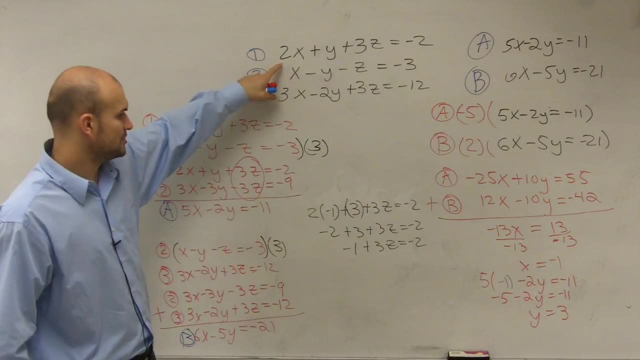 That becomes a negative. 1 plus 3z equals negative, 2. Add the 1, this negative: 1.. Whoa, whoa, whoa. what did I type in wrong 2 times? x is negative, 1. y is 3.. 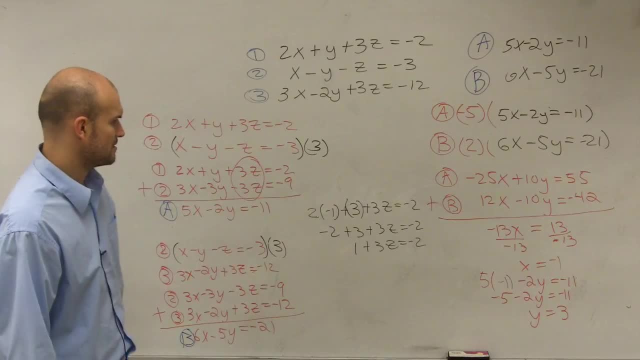 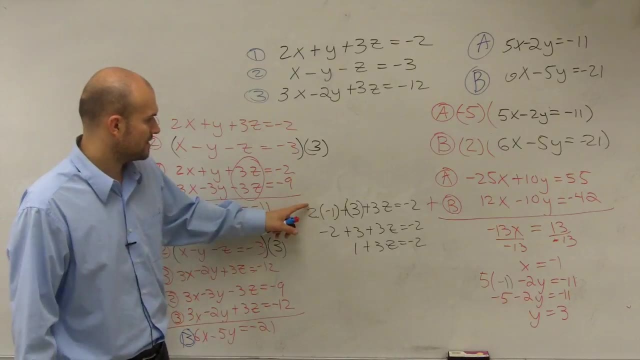 Oh, it's a positive 1, right. Where did I mess it up? There's something else I did wrong. Where's the negative 2?? Where did I type in wrong? Where am I writing in wrong? That's a negative 2, right. 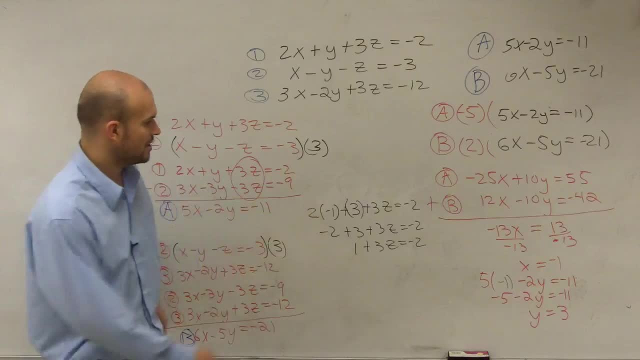 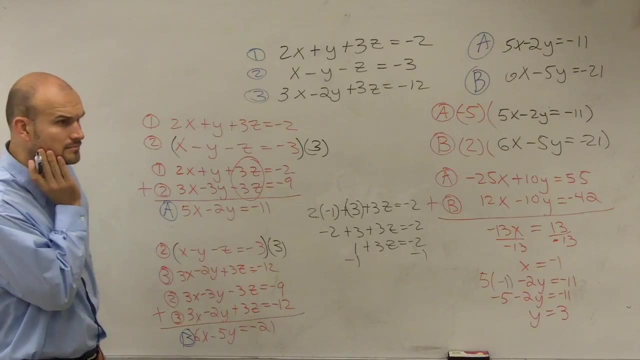 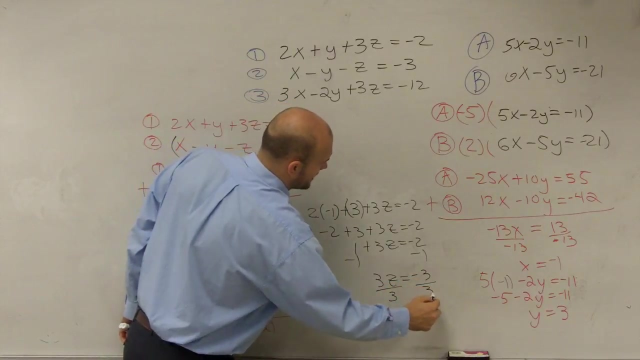 Right. Is that what you guys are talking about? No, okay, yeah, So there goes a positive 1.. So I subtract: 1. Right, 3z equals negative 3.. Divide by 3.. Therefore, z equals negative 1.. 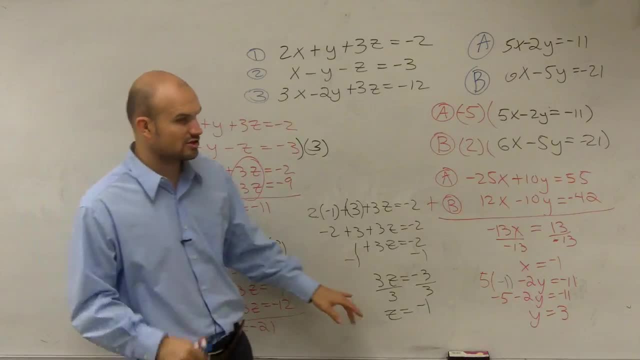 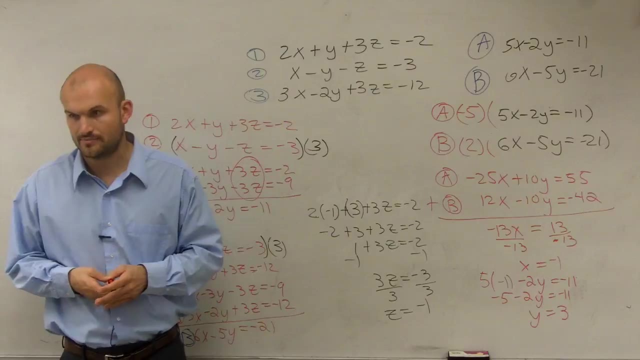 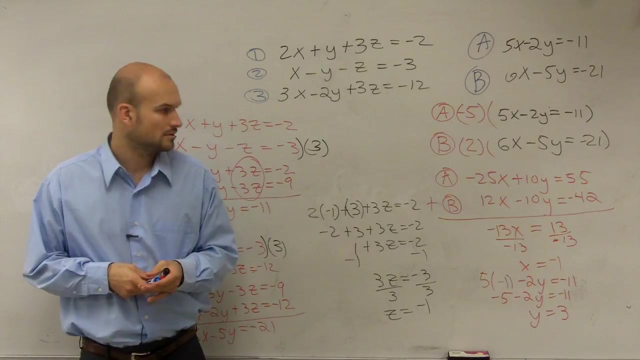 So, ladies and gentlemen, sorry, my final solution is going to be: z equals negative 1,, z equals or x equals negative 1, and z equals 3.. All right, And again, yes, Huh, Y was y. 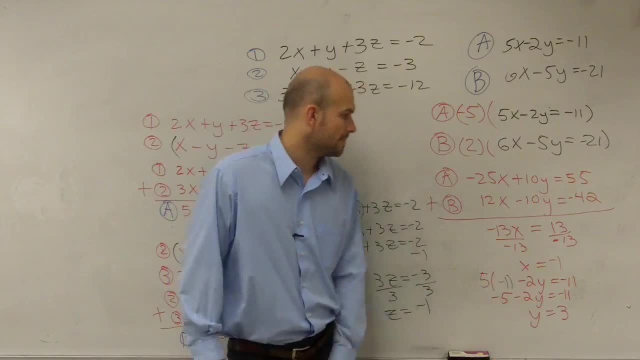 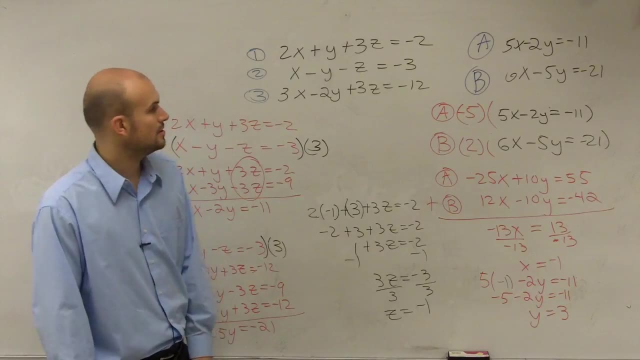 No, what is y? Y? Y is 3.. Up there, Okay, Yes, no, maybe so Good, Kevin, you can hit it if you like. Thank you.